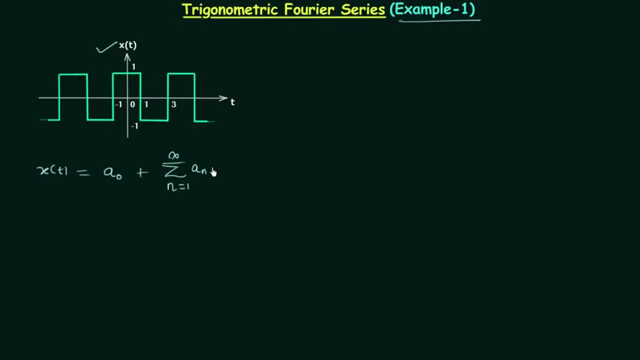 A sub n, which is the Fourier coefficient cos n, omega, naught t, plus all the sine terms. So n equal to 1 to infinity, Bn, which is another Fourier coefficient multiplied to sine n, omega, naught t. So this is the expansion, and now we will analyze the given signal. You can see, the given signal is symmetrical. 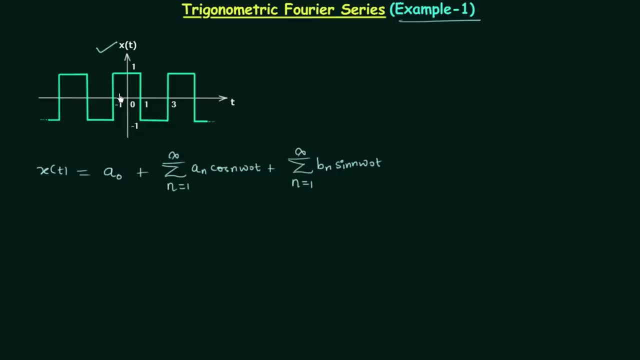 This is symmetrical about the time axis. This means when you calculate the area in one time period, you will find it is equal to 0. The positive area will cancel out the negative area and therefore we will have 0 as the total area in one time period. and therefore, when you calculate the average, when you divide the total area by the fundamental time period, you will find it is equal to 0.. So the average value or the DC value of this particular signal is equal to 0.. 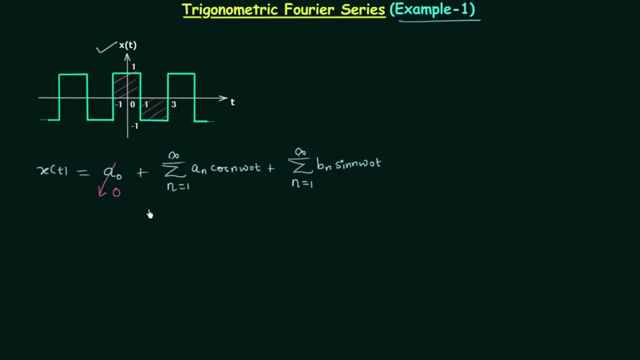 So we can say A naught is equal to 0.. So there is no need to calculate the A naught. Now you can see the given signal is also mirror image about the Y axis and when this happens the given signal satisfies the condition for even signals. This means when you perform the time reversal, when you find X minus T, you will find it is equal to XT. So when you fold the signal about the Y axis you will have 0.. 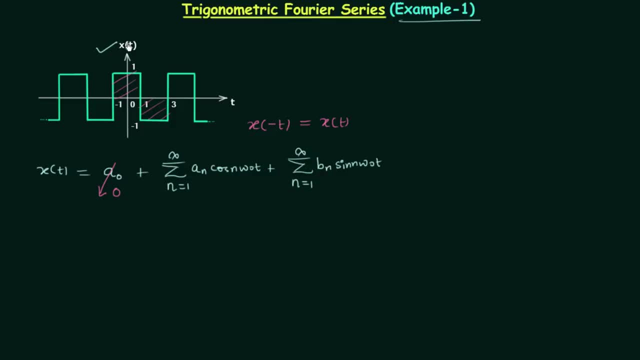 So we can say that we have the same signal and in that way we can say that XT is an even signal. and whenever we have even signal there is no need to calculate Bn, because there will be no sine terms. So Bn is also equal to 0 and thus there will be only cosine terms present in the expansion of signal XT. So we can rewrite the expansion like this: XT is equal to summation, n equal to 1, to infinity. 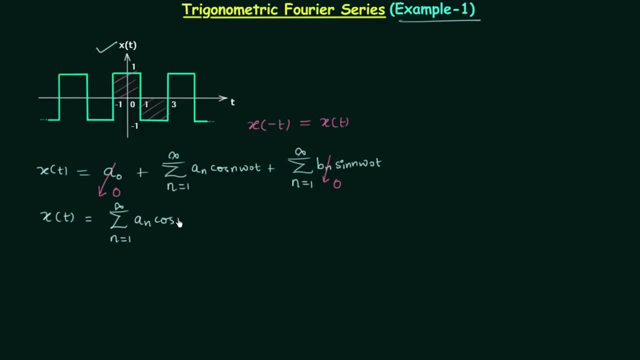 A sub n, cos n, omega, naught T. So our main task is to calculate this coefficient, an. Once we have an, we can substitute it in the expansion and we will have the Fourier series. expansion of signal XT. So I hope you now understand what is the use of analyzing the given signal before performing the calculations. Even if you perform the calculation for A naught, you will find it is equal to 0.. 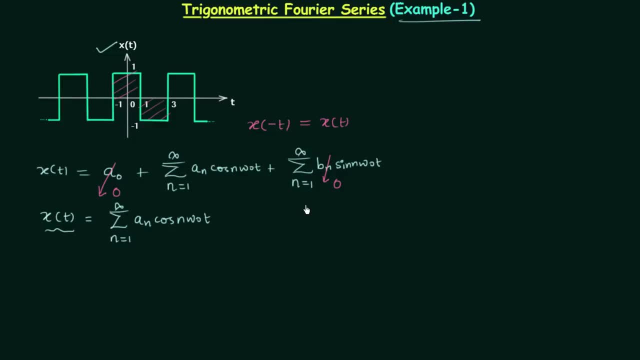 So you will end up wasting your time. The same thing goes for Bn. in this case, When you calculate Bn, you will find it is also equal to 0. So always try to analyze the given signal before performing the calculations. Now we will move on to calculation of an. We already know the formula for an. It is equal to 2 over fundamental time period: T naught integration signal: XT multiplied. 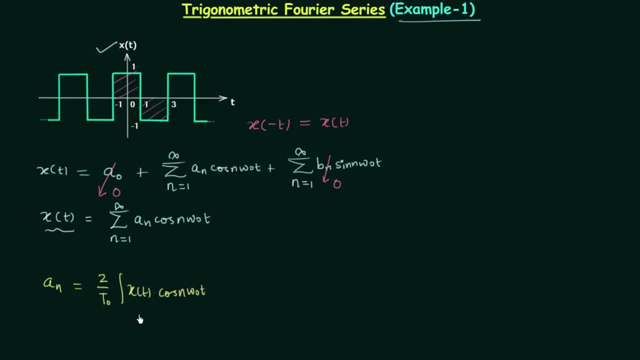 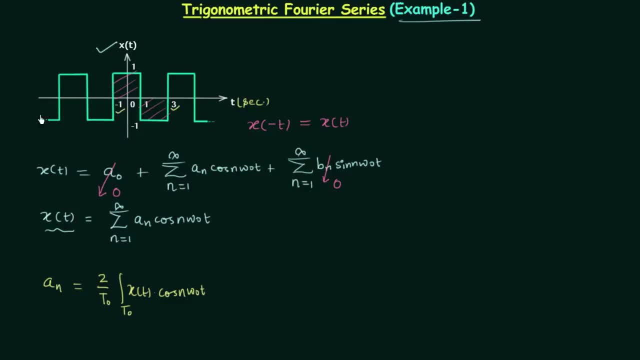 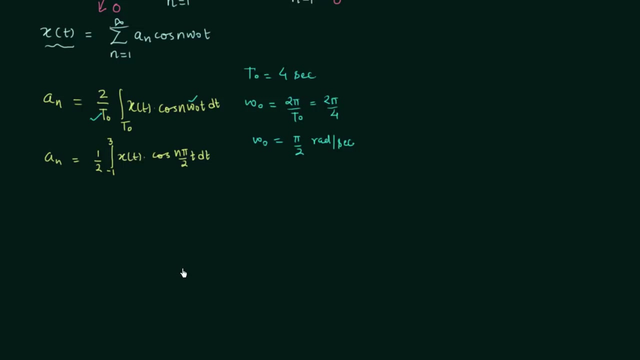 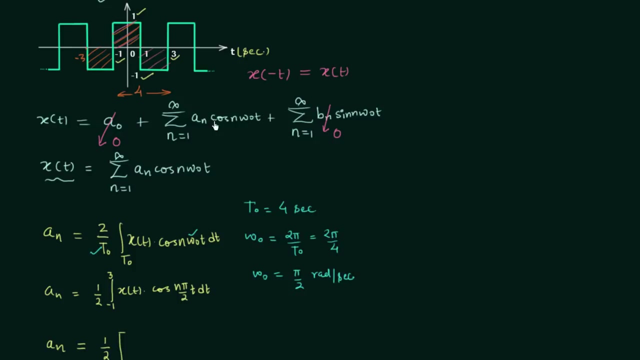 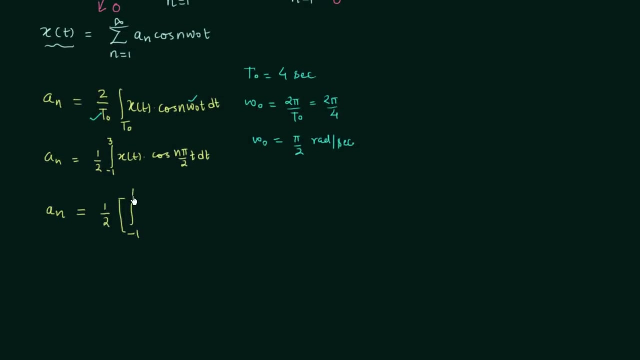 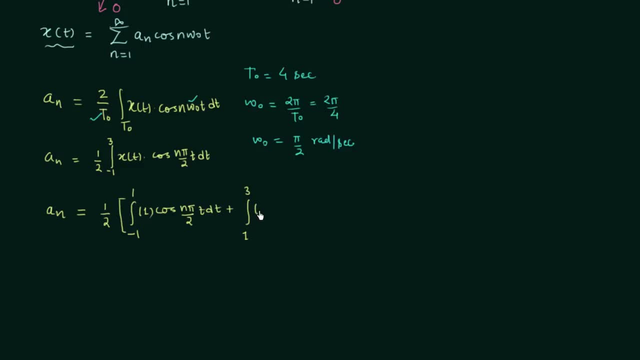 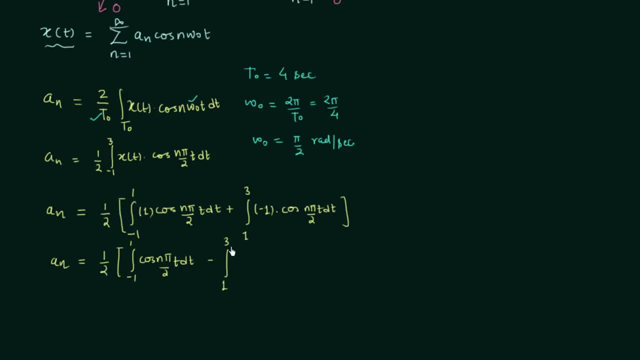 I have taken out integration 1 to 3 cos n pi by 2 t dt. Now we will assume n pi by 2 t as theta. To perform the integration, we will assume n pi by 2 t, equal to theta, and to find out: 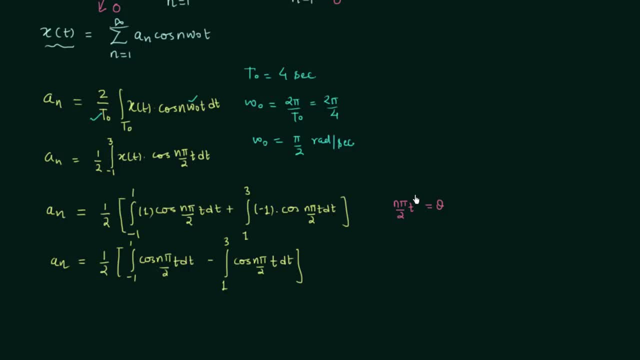 the very small value of theta. we will focus on t because n? pi by 2 is a constant. So if we have n? pi by 2, very small t, we will get very small theta, which is d theta and from here we can say dt is equal to 2 over n pi d theta. 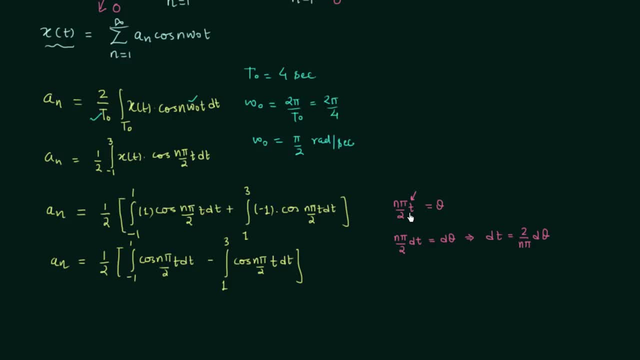 And as we are trying to have theta in place of n pi by 2 t, it is important to change the length of theta Because minus 1 here is the value of time t. So let's try to have theta when t is equal to minus 1, 1 and 3.. 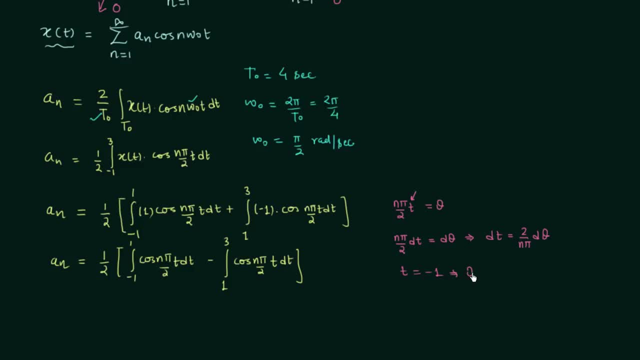 So when t is equal to minus 1, we have theta equal to minus n pi by 2.. Put t equal to minus 1 here and you will have theta equal to minus n pi by 2.. In the same way, when t is equal to 1, we have theta equal to n pi by 2.. 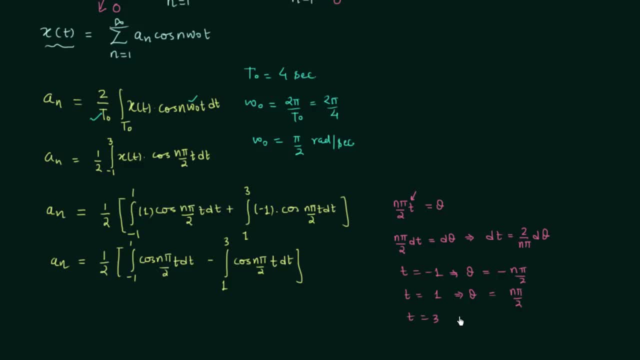 And when t is equal to 3, theta is equal to 3 n pi by 2.. Now we will substitute all these values in the integration. an will be equal to 1 by 2 integration. In place of minus 1, we will have minus n? pi by 2.. 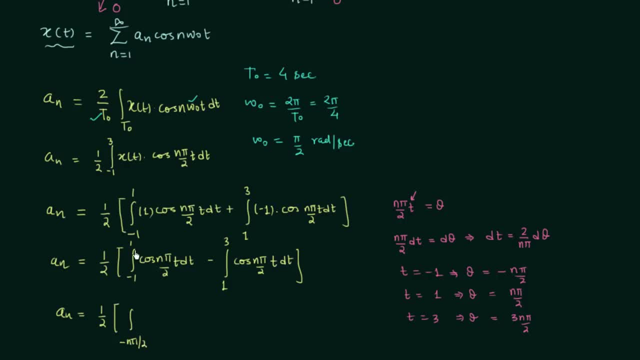 So we have minus n pi by 2.. In place of 1 we will have n pi by 2.. So that's n pi by 2.. n pi by 2 cos n pi. t by 2 is equal to theta. so we have cos theta and dt is equal to 2 by n pi. 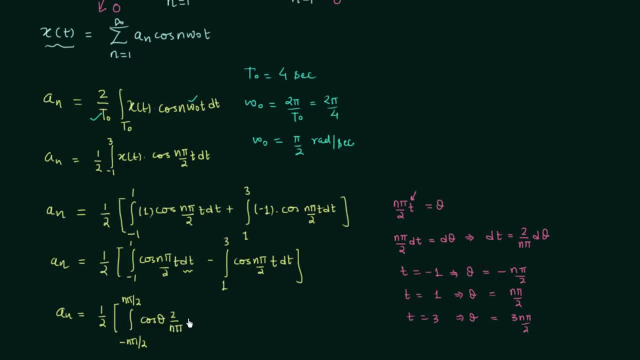 d theta, so 2 by n pi d theta. Similarly we have integration: n pi by 2 to 3, n pi by 2, cos theta 2 over n pi d theta, 2 over n pi is a constant, so we will take it out of integration. 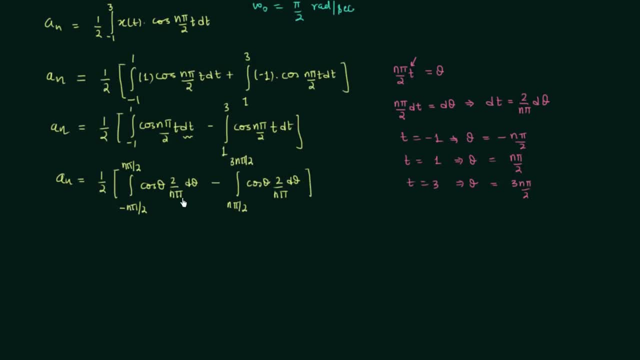 and 2 over n pi is common in both integrals. so we have an equal to 1 by 2 multiplied to 2 over n pi, which is the common term in both the integrals, and inside the bracket we have integration minus n pi by 2.. 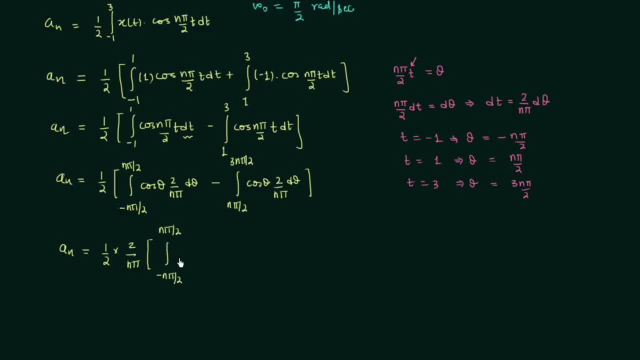 integration: n pi by 2 inches cos theta d theta. minus integration n pi by 2 to 3: n pi by 2 cos theta d theta. and we already know the integration of Cos. integration of Cos is equal to sine and differentiation of Cos is equal to minus sine. so integration of cos, 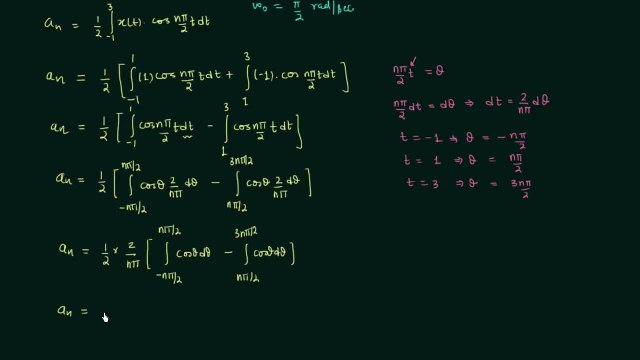 theta is equal to sine theta, So we have an equal to 1 by 2, pi by 2.. That's it. so that's all by n pi. This 2 and 2 will cancel out, So we have 1 over n pi. Integration of cos theta. 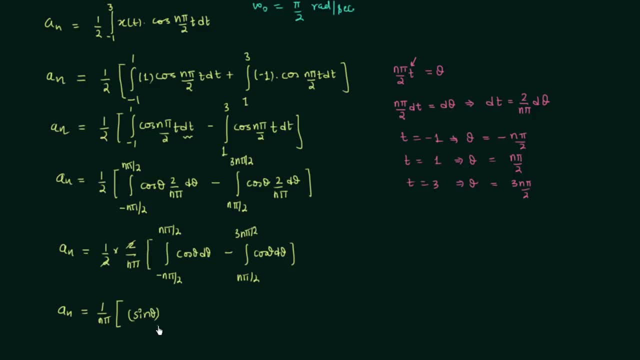 is sine theta. The lower limit is minus n pi by 2 and the upper limit is n pi by 2.. And again, the integration of cos theta is equal to sine theta. The lower limit is n pi by 2 and the upper limit is 3 n pi by 2.. Now we will put the lower and upper limits. 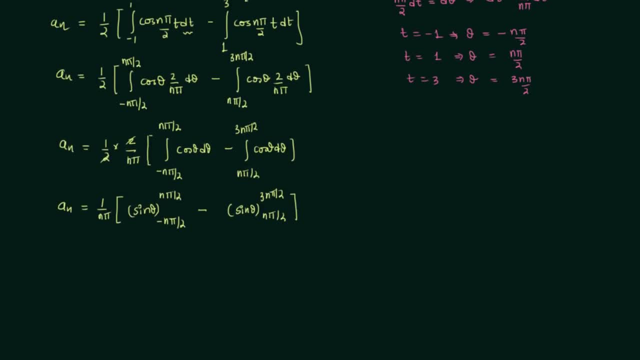 and we will see what we have. First we will deal with the result from the first integral and we will have sine n pi by 2, sine n pi by 2 by putting the upper limit. Then we have minus sine, minus n pi by 2.. 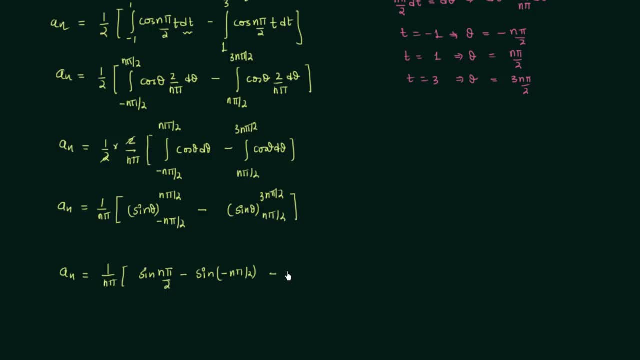 Then we have sine 3 n pi by 2, sine 3 n pi by 2, and then we have minus sine n pi by 2.. And because of this minus, this minus will become plus. So this is what we have In place. 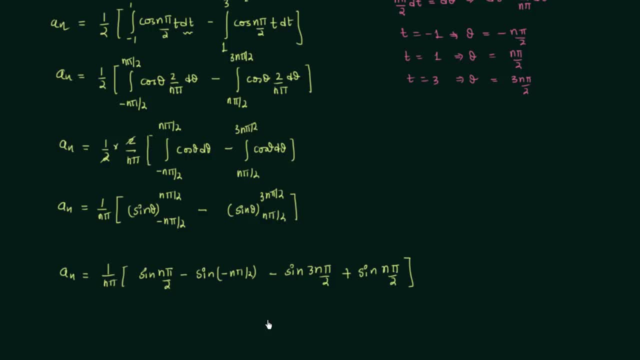 of theta. we have substituted the upper and lower limits. Now we will focus on the middle 2 terms. We will focus on Sine minus n pi by 2. by 2 and sine 3n pi by 2.. So first we will talk about sine minus n pi by 2.. For this you should 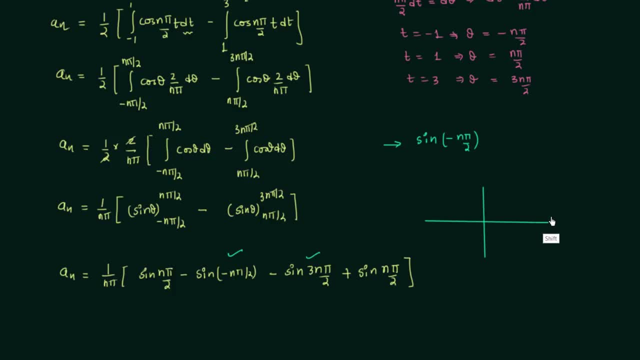 know about the basics of trigonometric ratios. This is 0 degree, 360 degree, this is 90 degree, this is 180 degree and this one here is 270 degrees. This is the first quadrant, this is the second quadrant, this is the third quadrant and this one here is the fourth quadrant. 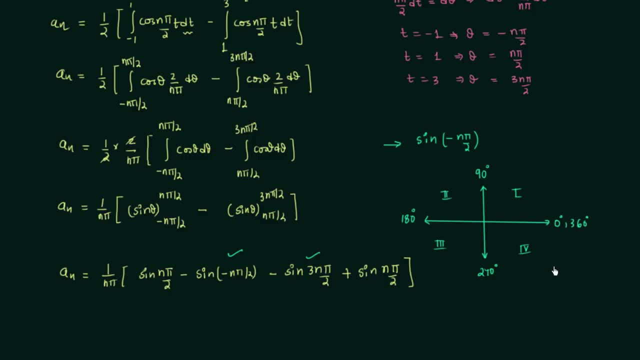 In first quadrant all the trigonometric ratios are positive, So I will write, I will write all in the first quadrant. In the second quadrant, sine and cosec are positive, So I will write sine here. In the third quadrant, tan and cote are positive, So I will write tan here and 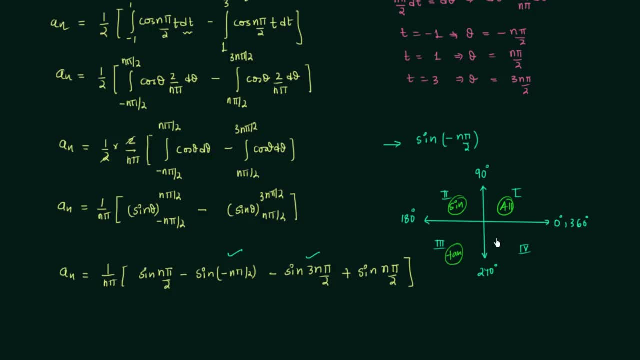 in the fourth quadrant, cosec and sec are positive and you can remember it as all silver tea cups. To understand this, I will take one example. In this example we have sine pi by 2, minus theta. Pi by 2 means 90.. 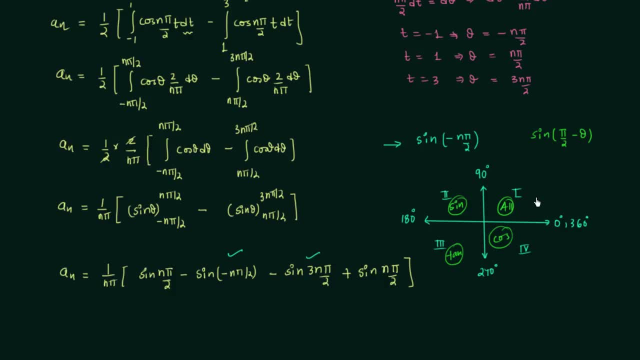 So we have 90 minus theta. 90 minus theta means we are in first quadrant. So the sign we are going to get is positive because in first quadrant all the ratios are positive. Now, as we are having pi by 2 here, sign will change to cos. 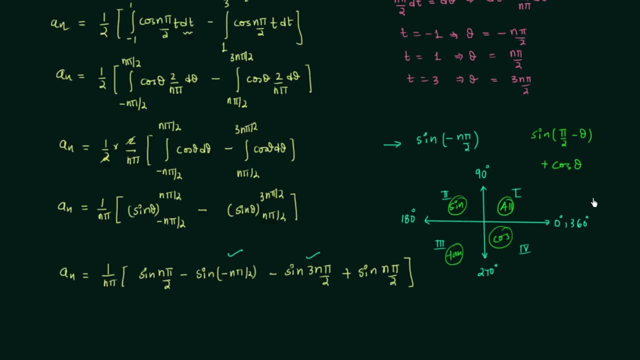 So we have cos theta, Very simple. Let's take another example. In this example I will take sign pi minus theta. Pi minus theta means we are in the second quadrant. 180 minus theta is between 90 and 180 degrees. Therefore we are in second quadrant and in second quadrant sign is positive. 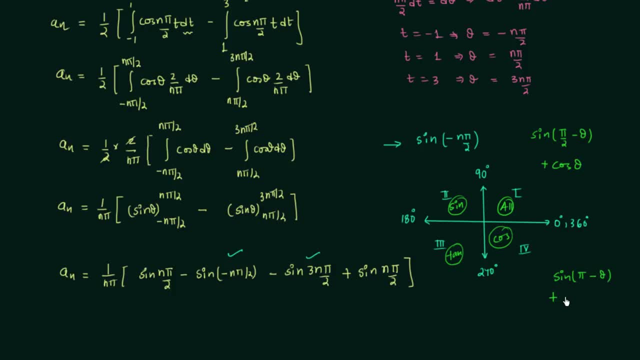 180 degrees plus minus anything. sign will not change to cos, It will remain sign. So we have sign theta. So sign pi minus theta is equal to plus sign theta. So in this way we have to use the quadrants and this shows the actual variation of signs. 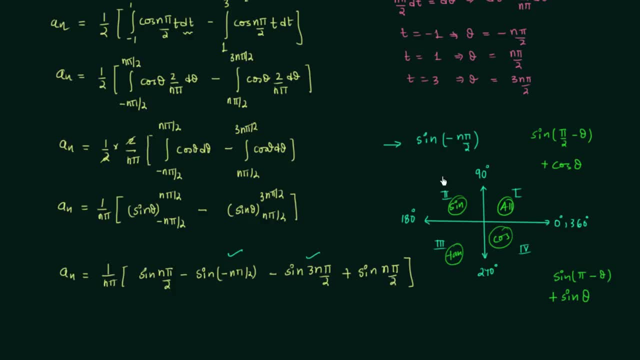 cos, etcetera. with change in angle, Now we will focus on sign minus n pi by 2.. I can write sign minus n pi by 2 as sign zero minus n pi by 2.. Zero minus something will lie in fourth quadrant, and in fourth quadrant cos is positive and 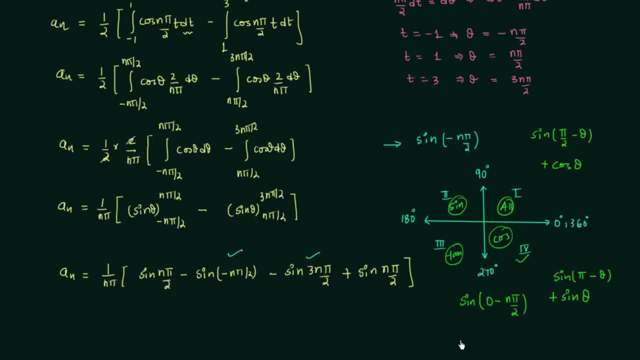 sec is positive, But here we have sign, So we have negative sign And as we are having zero minus something, Sign will not change to cos. So we have sign n pi by 2.. So overall we have minus sign n pi by 2 in place of sign minus n pi by 2.. 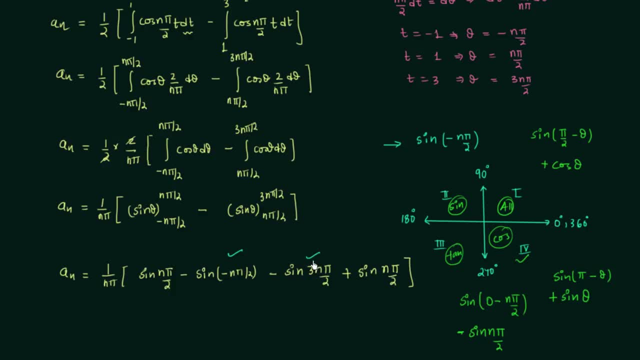 So we are done with the second term. Now we will focus on the third term, which is sign 3n pi by 2.. I will change the color of my pen. Here we have sign 3n pi by 2.. I can write it as n pi plus n pi by 2.. 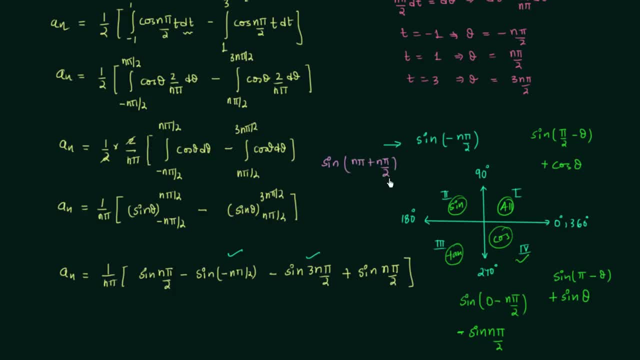 So we have negative sign minus sign n pi by 2.. So we have negative sign minus sign n pi by 2.. This is also negative sign minus sign n pi by 2. Which is nothing but sign 3n pi by 2.. 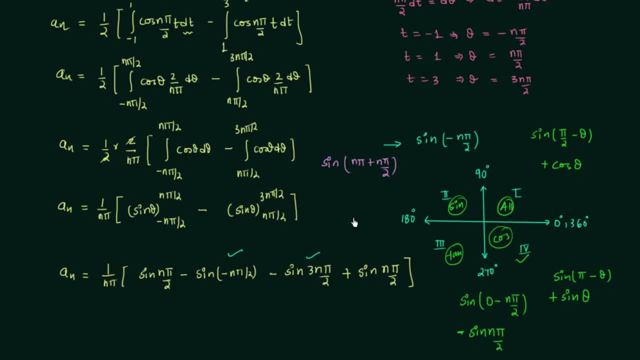 Now, when n is even, we have some different result. When n is odd, we have some different result. So we have to focus on two different cases. In case number one, when n is even, n pi means 360 degrees. For example, when n is 2, we have 2 pi, which is 360 degrees. 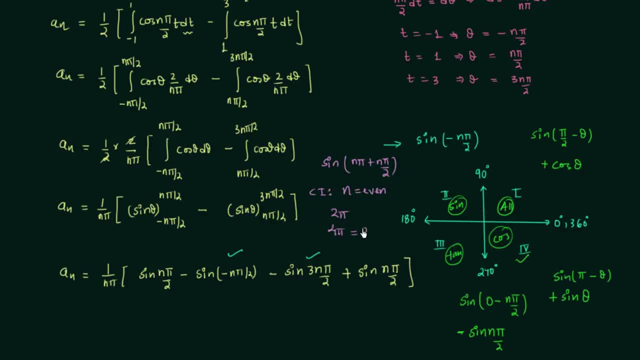 When n is 4, we have 4 pi, Which is nothing but 2 times 360 degrees. so it means two revolution, and again you are at 360 degrees. so when n is even, we are at 360 degrees, and 360 degrees plus something moves us in the first quadrant and in first 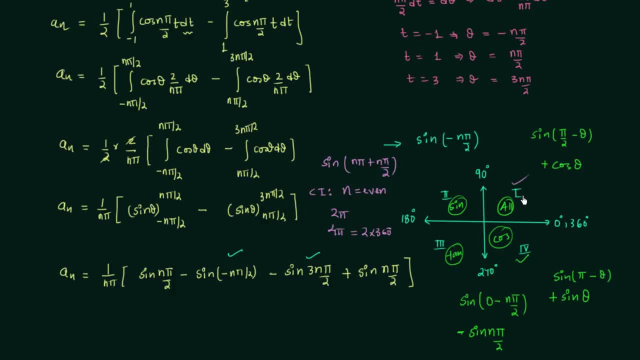 quadrant. every trigonometric ratio is positive. so we have sine and pi by 2. sine will not change to cause because we are at 360 degrees. sine will change to cause only when we have 90 degrees plus minus something or 270 degrees plus minus something. so when n is even in place of sine 3 and pi by 2, 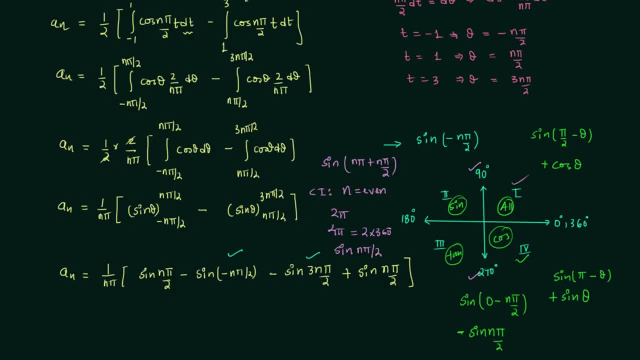 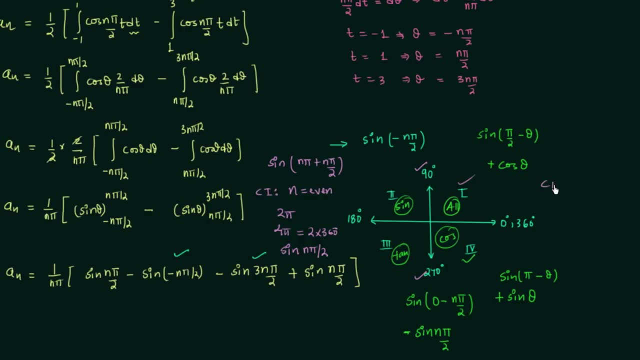 we can have sine and pi by 2. now we will discuss the next case, case number 2, in which we will consider n to be odd. so I am writing case number 2 here. in this case, n is odd. when n is odd, let's take one example. let's say n is equal to 1, we have sine pi plus pi by 2. pi means 180 degrees. 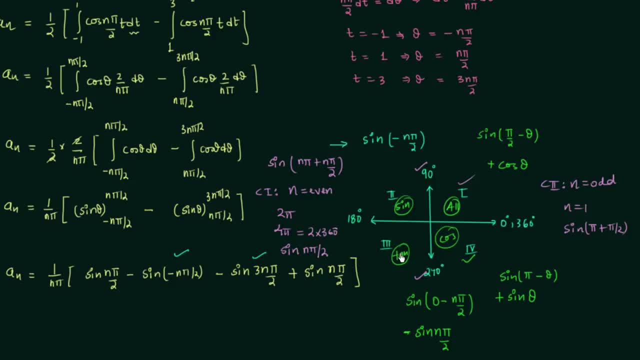 and 180 degrees plus, something moves us in the third quadrant, and in third quadrant sine will become negative. however, sign will not change to cause. so we have minus sine and pi by 2. so when n is odd, we have minus sine and pi by 2, and pi by 2 we have minus sine and pi by 2. so we have: 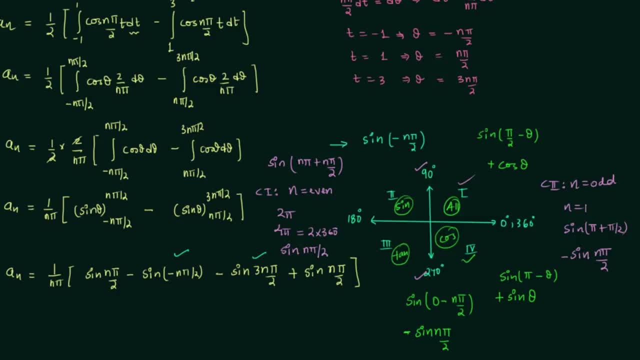 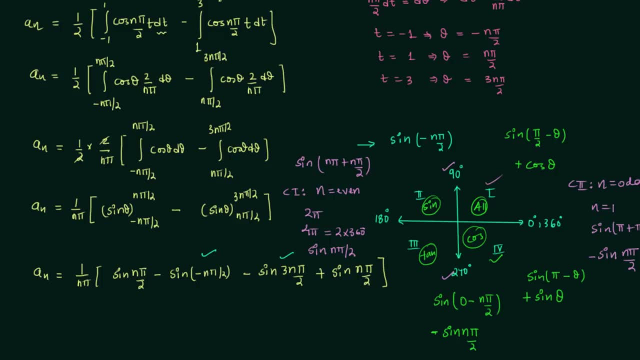 in place of sine 3n pi by 2.. Considering these two important points, we will write down an, and this time we will write it down for two different cases. In case number one, we have considered n to be even, so we have an equal to 1 over n pi inside the bracket. 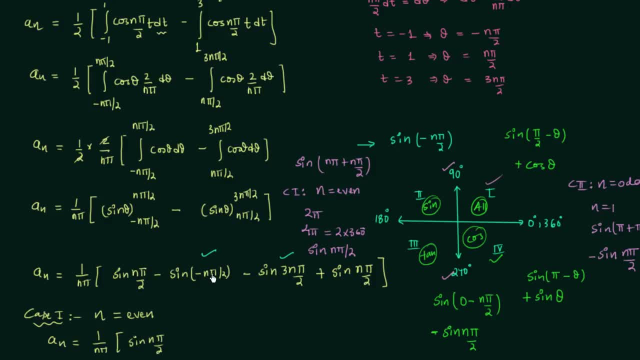 sine n pi by 2.. In place of sine minus n pi by 2, we have minus sine n pi by 2.. This negative sine was already there, so we have plus sine n pi by 2.. In place of sine 3 n pi by 2, we can. 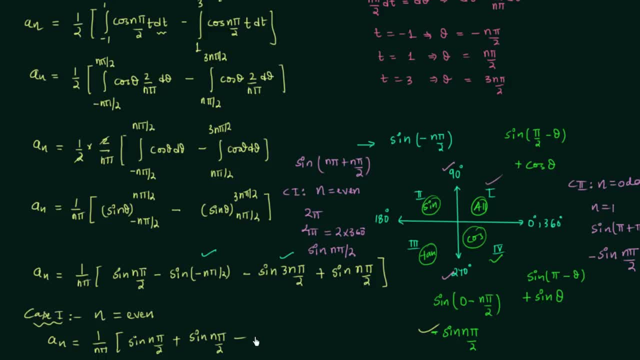 write sine n pi by 2.. Negative sine was there, so we have minus sine n pi by 2 and this sine n pi by 2 will come as it is. So you can see, we have sine n pi by 2 cancelled out and we are left with 2 times sine n pi by 2 multiplied. 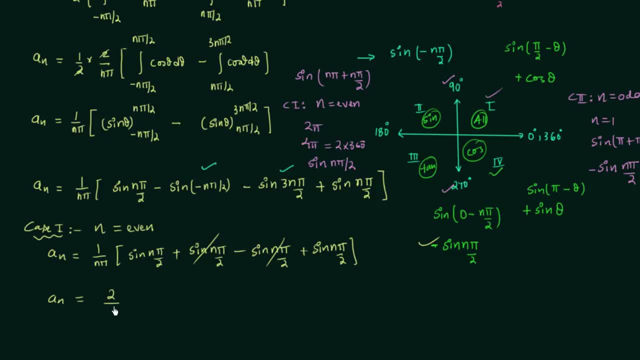 to 1 by n pi. So an is equal to 2 over n pi, sine n pi by 2.. Now again, you have to focus on very important point here. n is even now. try putting something even here. For example, let's take n equal to 2.. Let's take n equal to 2. this will give: 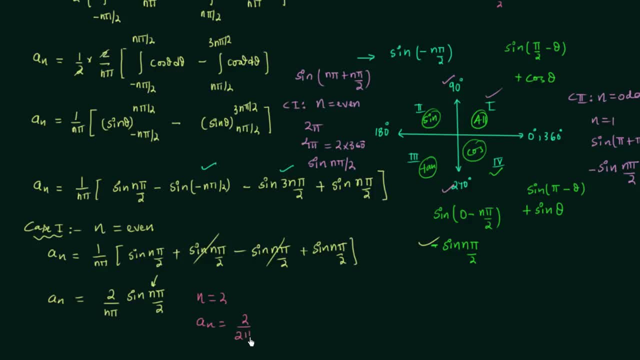 us an equal to two over two pi sine two pi by two. or we can write: an is equal to one over pi sine pi. Sine pi is equal to zero. or you can say: whenever you have sine n pi, it is going to be zero, and whenever you put n something, even, you will get the integral. 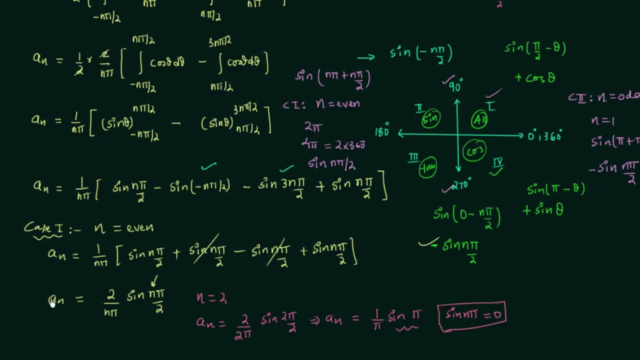 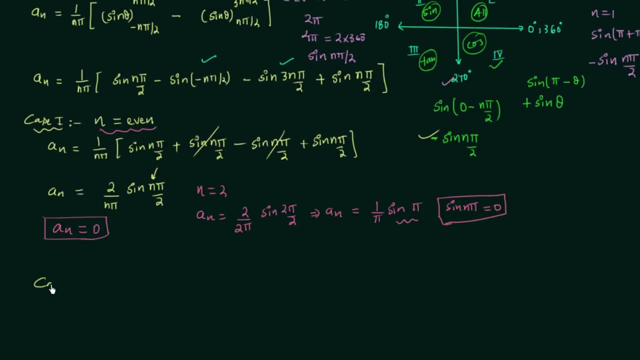 multiple of pi. So every time you are going to get a n equal to zero if n is even. So, a n is equal to zero when n is even. Now we will consider the case number two, in which n is odd. So let's move to case number two, and in this case n is odd For odd. we have 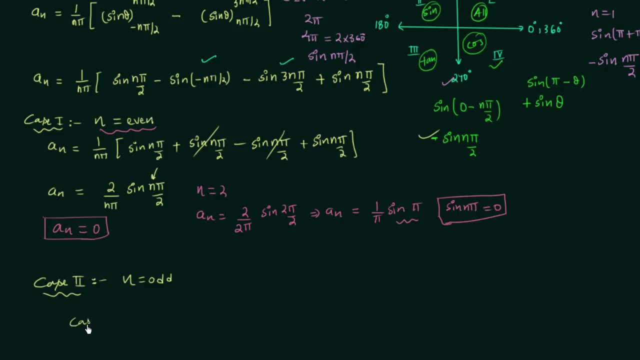 again two different cases. Let's the first case, case A. In this case, N is 1, 5,, 9,, 13 and so on, And in case B, N is equal to 3,, 7,, 11,, 15 and so on. I will explain why we have taken two different cases when 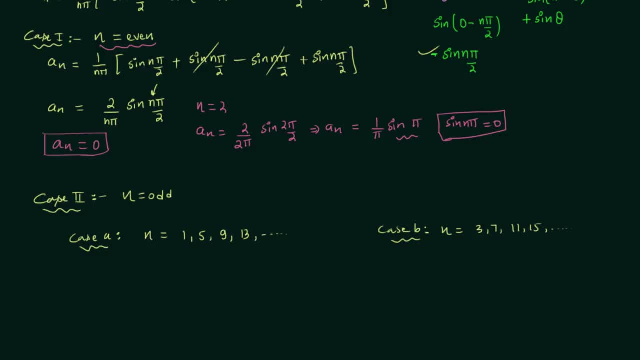 N is odd. Let's discuss the first case, when N is 1,, 5,, 9,, 13 and so on. In this case, A will be equal to 4 over N pi. It is equal to 4 over N pi because we can clearly. 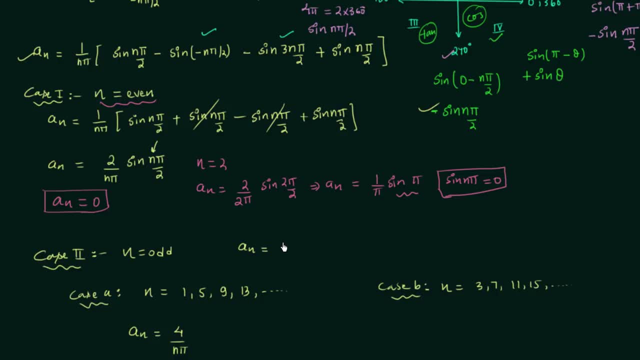 see from here: A is equal to 1 over N pi, sine N pi by 2, sine N pi by 2, sine minus N pi by 2.. It is equal to minus sine N pi by 2.. Negative sine was already there, so we have sine N. 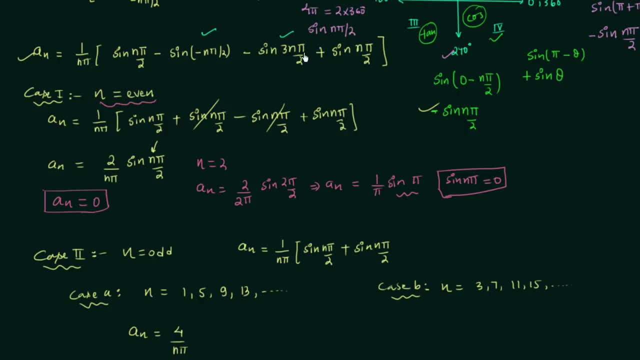 pi by 2.. Now there is difference if you compare the third term in case of even and in case of odd. In case of odd, we have sine 3 N pi by 2 equal to minus sine N pi by 2.. Minus: 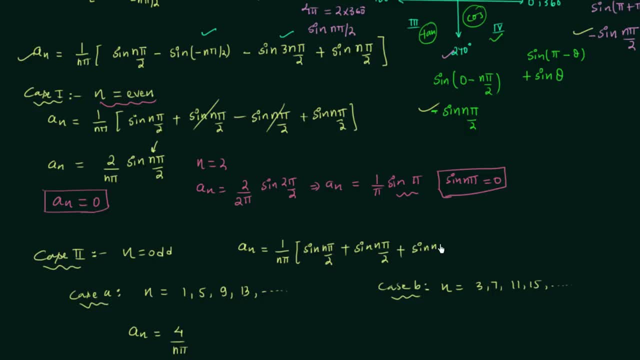 sine was already there, so we have plus sine N pi by 2. And this term will come as it is: sine N pi by 2.. So from here, An is equal to 4 times sine N pi by 2, multiplied to 1 by N pi, Or we can: 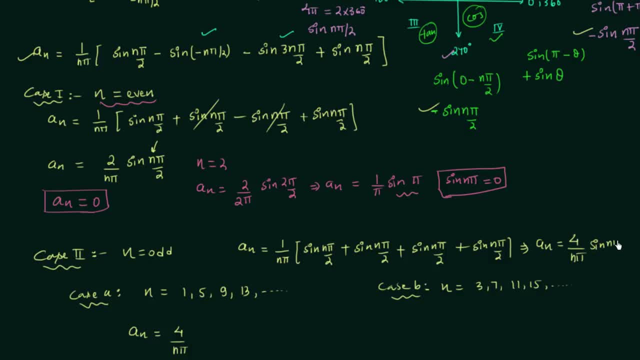 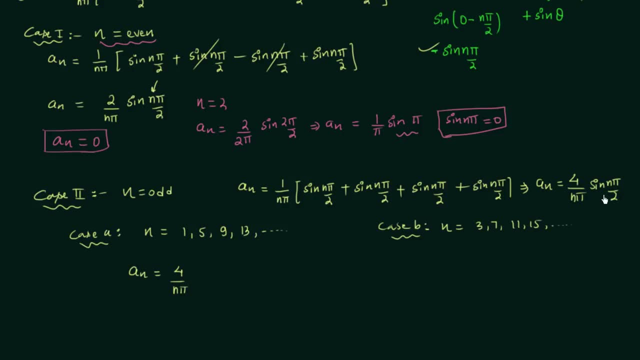 write 4 over N pi, sine N pi by 2.. And when N is 1,, 5,, 9,, 13 and so on, we will have sine N pi by 2 equal to plus 1, because we know sine pi by 2 is equal to plus 1.. But sine. 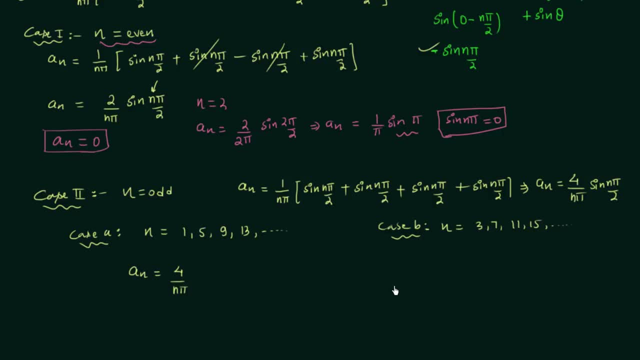 3 pi by 2 is equal to minus 1.. And the same way the cyclical equation can be used to: the cycle will repeat itself. So whenever we have 1,, 5,, 9,, 13 and so on, this sine n. 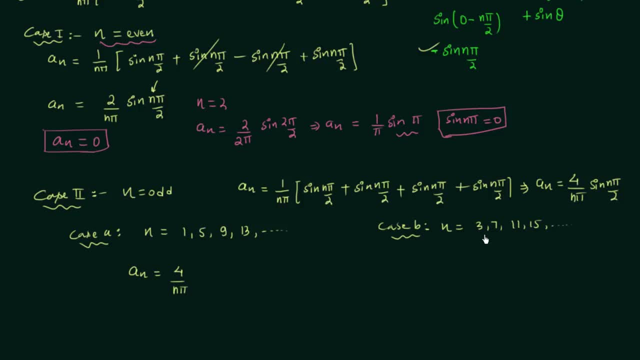 pi by 2 will become plus 1, and whenever we have n equal to 3,, 7,, 11,, 15, this sine n pi by 2 will become minus 1.. So a n will be 4 by n pi for this case and a n will be. 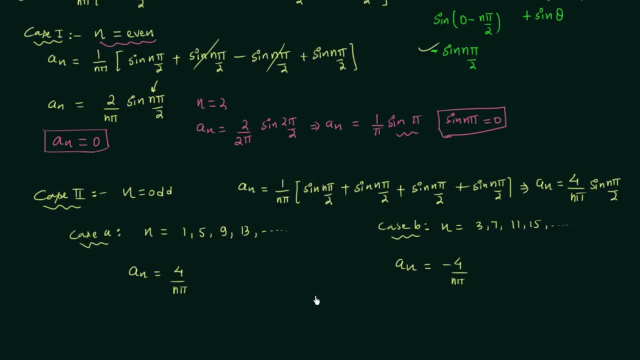 minus 4 over n pi for this case. So we have everything to substitute in our expansion and after analyzing the given waveform, we have seen a naught and b, n is equal to 0. So x, t is equal to summation, n equal to 1, to infinity. a n, cos, n, omega, naught, t, omega. 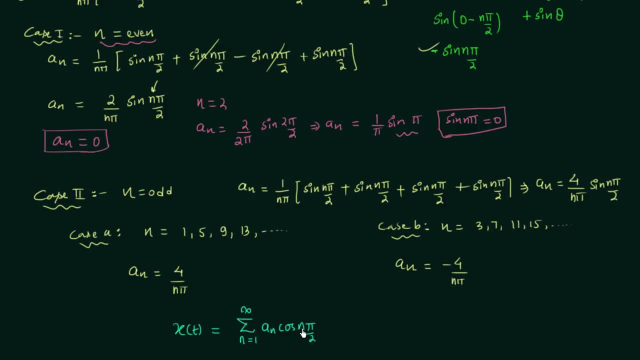 naught is equal to pi by 2.. So we have cos n, pi by 2 t. Now we will expand it by putting the different values of n First. we will find out the value when n is equal to 1.. So this, yes, we will find the value by putting the different values of n. 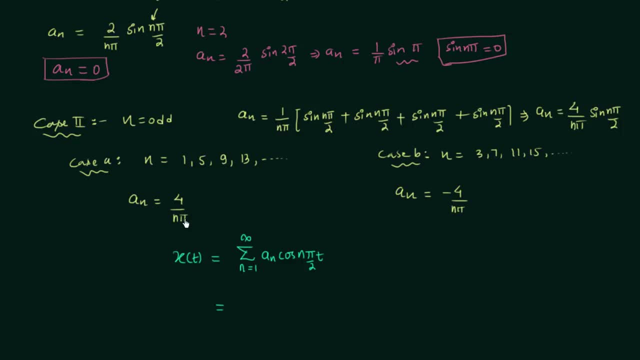 1. When n is equal to 1, a n is equal to 4 by n, pi n is equal to 1.. So it is good to call a n as a 1, and a 1 is equal to 4 by 1 into pi, So 4 by pi, and here we have cos. 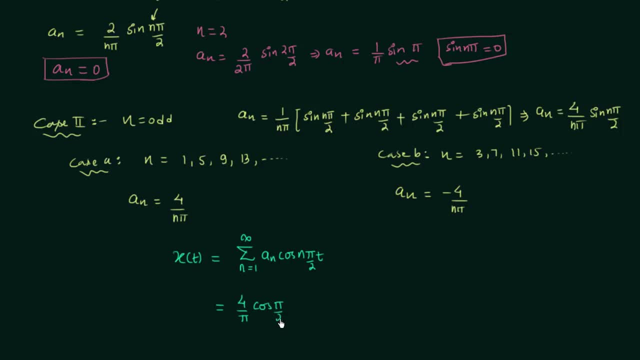 pi by 2 t, cos pi by 2 t. After this we will find out the value when n is equal to 2.. When n is equal to 2, we have already seen a n is equal to 0, because n is even So 0 multiplied. 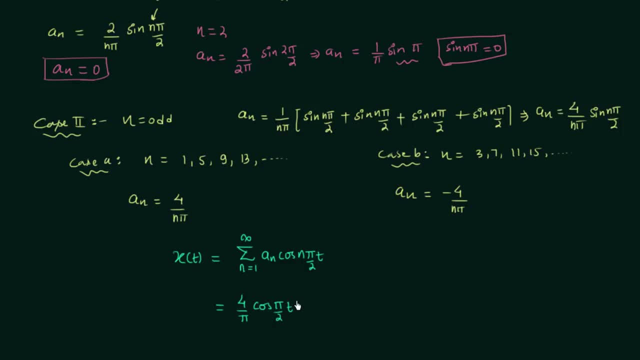 to cos pi, t will be equal to 0. So we will only focus on the odd values from now. So when n is equal to 3, you can see a n is equal to minus 4 by n pi, and as n is equal to 3,. 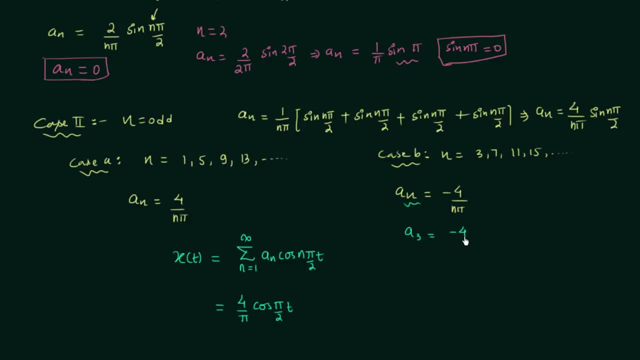 it is good to call a 3, and it is equal to minus 4 by 3 pi. So here we have minus 4 by 3 pi 5. and cos n pi by two t will be cos three by two pi t. 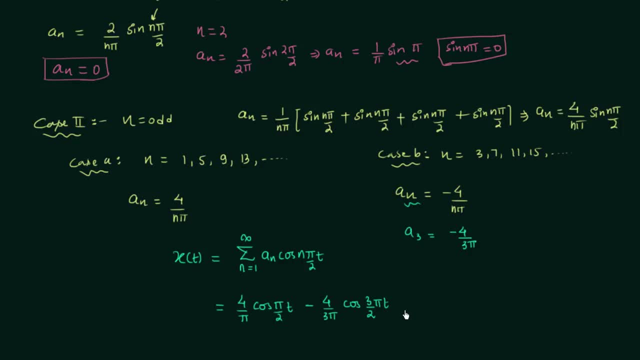 In the same way we will find out the value. when n is equal to five, It is equal to plus four by five pi cos five pi by two t. And when n is equal to seven, we have minus four over seven pi cos seven pi by two t. 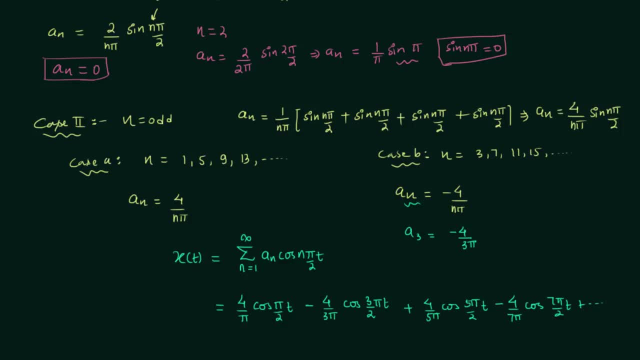 and so on. You can see four by pi is common in all the terms. So we will take four by pi common and inside the bracket we will have cos pi by two t minus one by three. cos three pi by two t plus one by five. cos five pi by two t. 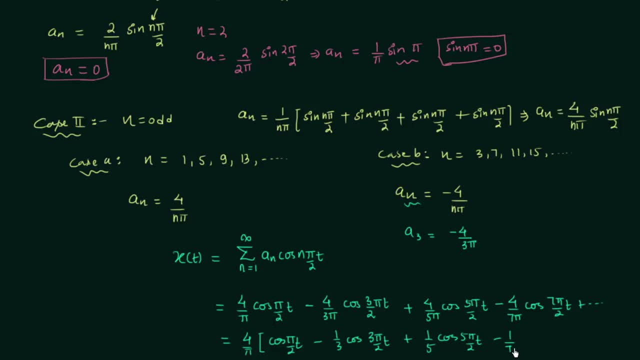 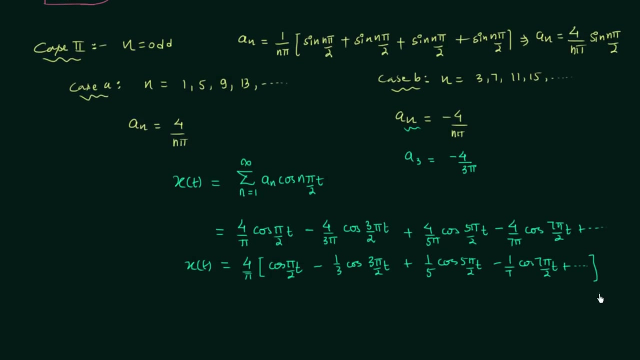 After this we have minus one by seven, cos seven, pi by two, t And so on. So this is our answer. This is the expansion of signal xt using the trigonometric Fourier series expansion, And you can see we have different harmonics. 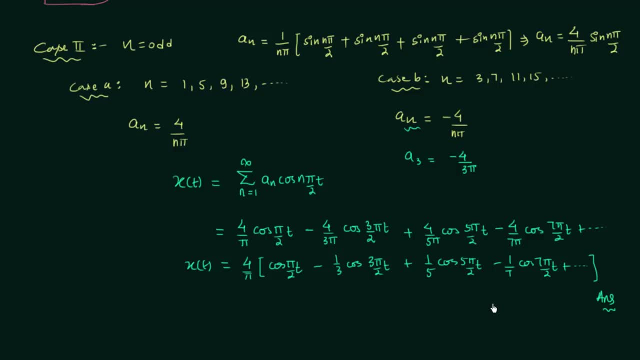 in this expansion. So this is the complete process to find out the trigonometric Fourier series expansion. The only important thing is the integration. You can see, if you do not know how to perform the integration, you cannot have this result. So this is all for this lecture. 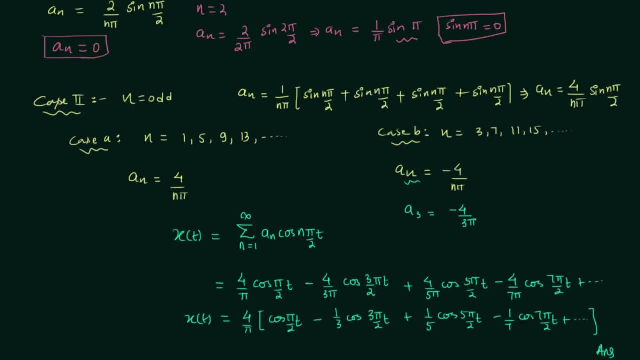 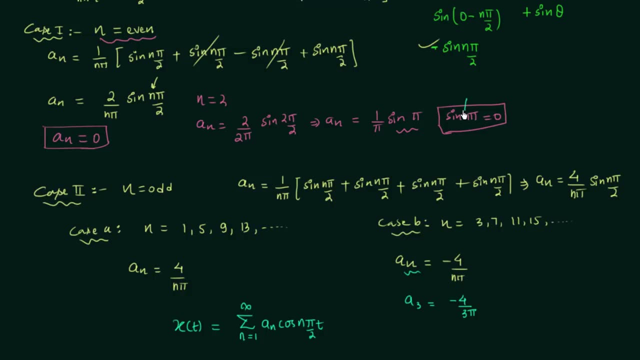 There is one thing I want To change here. If you remember, I told you, whenever we have integral multiple of pi, sine will become zero. I have used n here, which I don't want to use. I will use m in place of n.